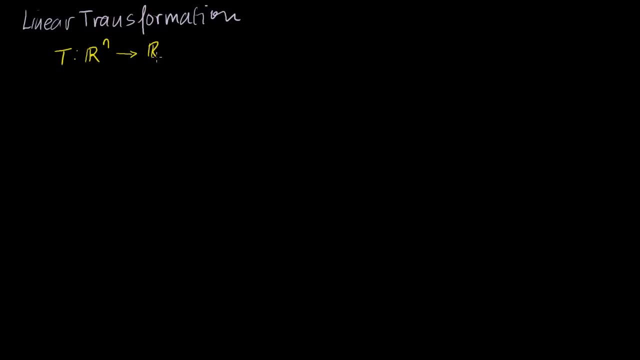 next video why I'm being a little bit particular about that, although they are just arbitrary letters Where the following two things have to be true. So if something is a linear transformation, if, and only if the following thing is true: Let's say that we have two vectors. 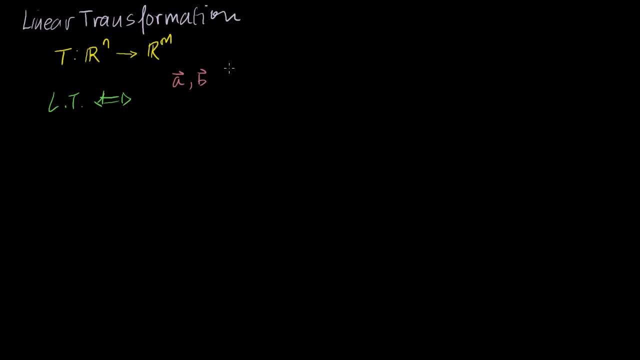 Say, vector a And let's say vector b are both members of Rn, So they're both in our domain. So this is a linear transformation. if, and only if, I take the transformation of the sum of our two vectors, If I add them up first, that's equivalent to taking the. 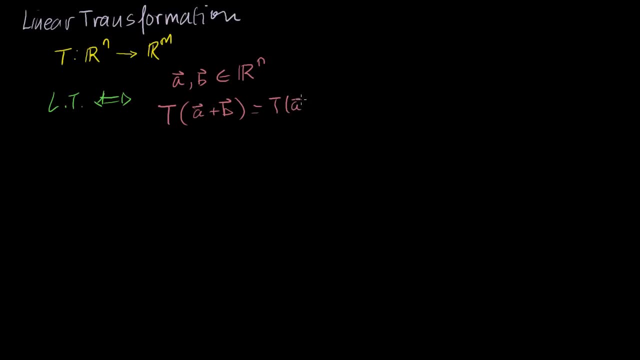 transformation of each of the vectors and then summing them. That's my first condition for this to be a linear transformation. And then the second one is: is that if I take the transformation of any scaled up version of a vector, So let me just multiply vector a times some real number, c. 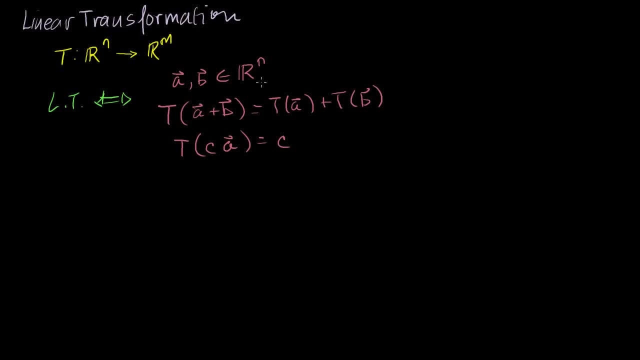 If this is a linear transformation, then this should be equal to c times the transformation of a. That seems pretty straightforward. Let's see if we can apply these rules to figure out if some actual transformations are linear or not. So let me define a transformation. 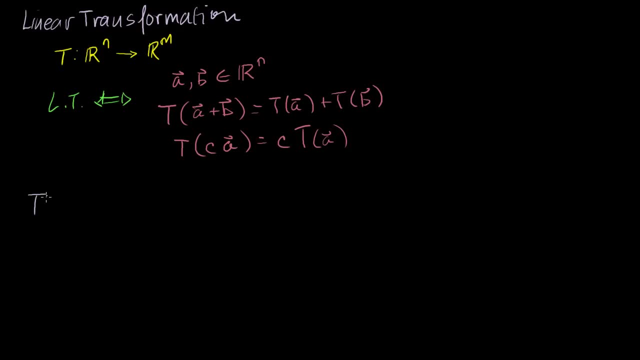 Let's say that I have the transformation t Part of my definition. I'm going to tell you It maps from R2 to. let's do something. let's just say it maps from R2 to R2.. And it maps. So if you give it a two-tuple right, its domain is two-tuple. 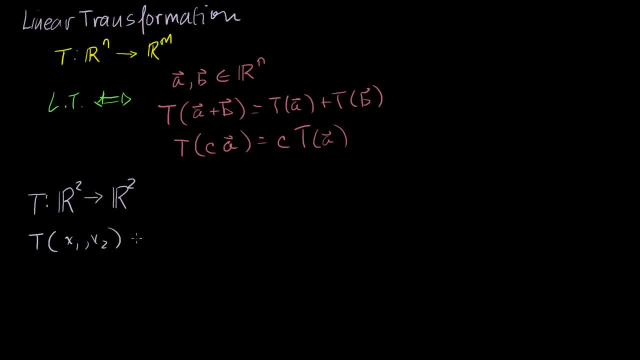 So you give it an x1 and an x2.. Let's say it maps to, so this will be equal to or it's associated with. let me just say x1 plus x2.. And then let's just say it's 3 times x1 is the second tuple. 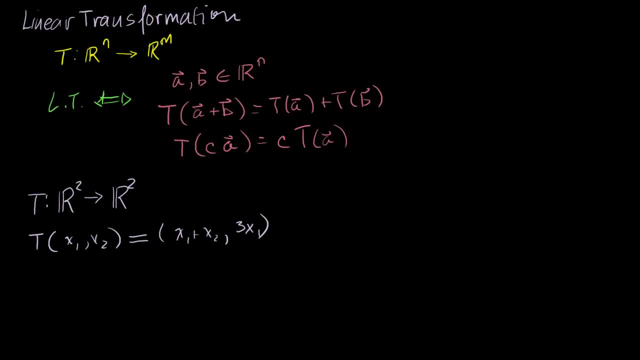 And we could have written this more in vector form. This is kind of our tuple form. We could have written it- and it's good to see all the different notations that you might encounter- You could write it that a transformation of some vector. 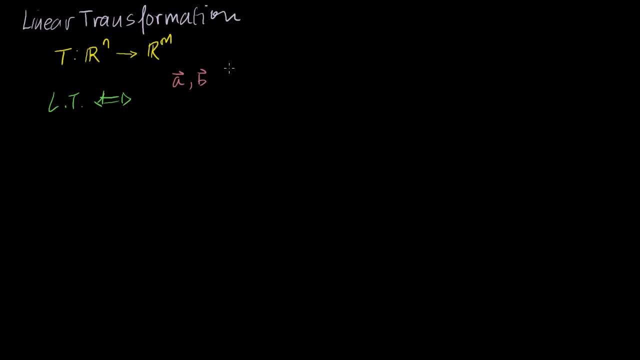 Say, vector a And let's say vector b are both members of Rn, So they're both in our domain. So this is a linear transformation. if, and only if, I take the transformation of the sum of our two vectors, If I add them up first, that's equivalent to taking the. 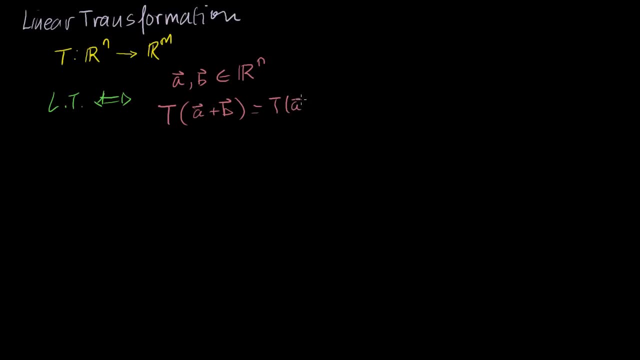 transformation of each of the vectors and then summing them. That's my first condition for this to be a linear transformation. And then the second one is: is that if I take the transformation of any scaled up version of a vector, So let me just multiply vector a times some real number, c. 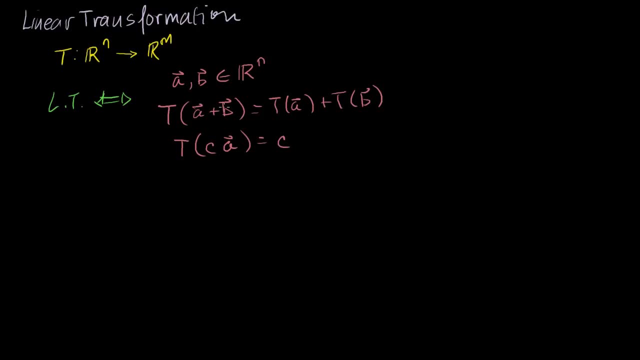 If this is a linear transformation, then this should be equal to c times the transformation of a. That seems pretty straightforward. Let's see if we can apply these rules to figure out if some actual transformations are linear or not. So let me define a transformation. 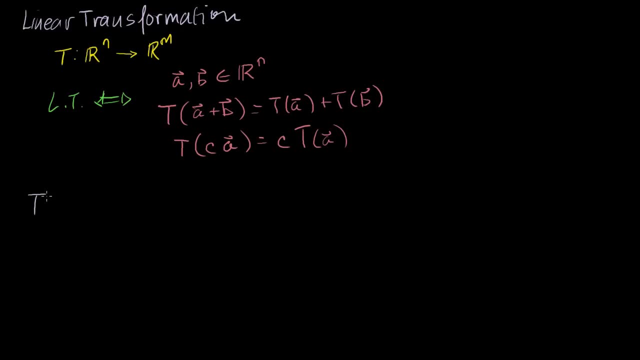 Let's say that I have the transformation T Part of my definition. I'm going to tell you It maps from R2 to. let's do something. let's just say it maps from R2 to R2.. And it maps. 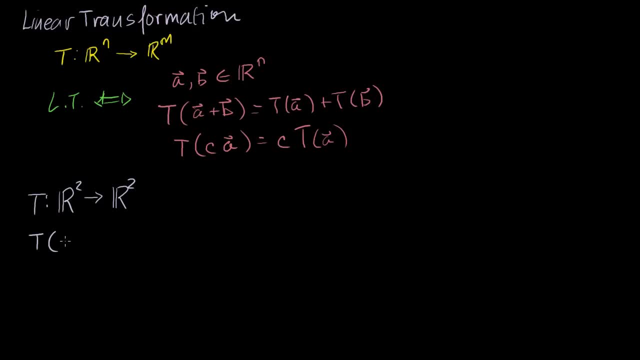 So if you give it a 2-tuple right, Its domain is 2-tuple. So you give it an x1 and an x2.. Let's say it maps to. so this will be equal to or its associated with, let me just say x1 plus x2.. 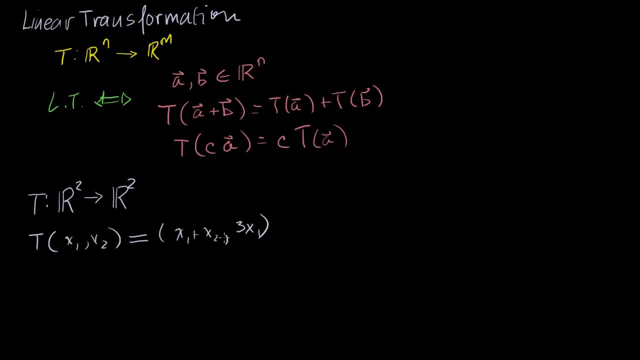 And then let's just say it's 3 times x1, is the second 2-tuple, And we could have written this more in vector form. This is kind of our tuple form. We could have written it and it's good to see all the 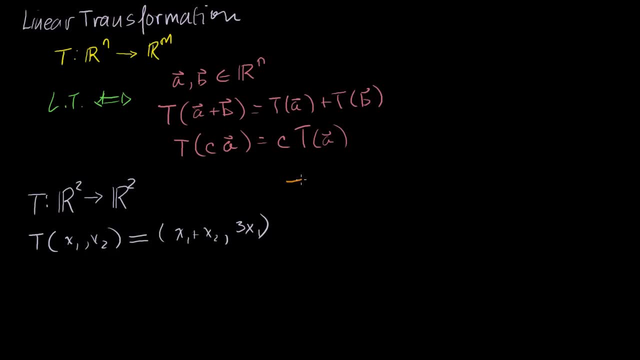 different notations that you might encounter. You could write it that a transformation of some vector x, where the vector looks like this: x1, x2.. Let me put a break, Let me put a bracket there. It equals some new vector x1 plus x2, and then the second. 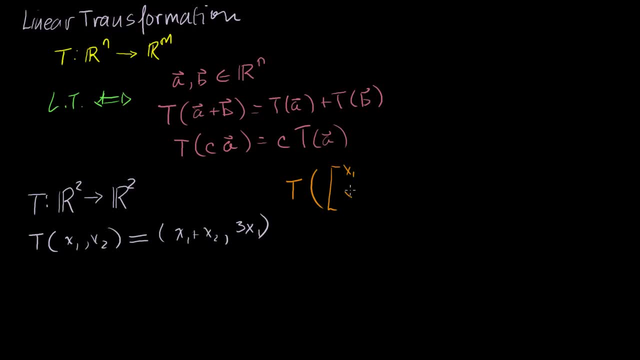 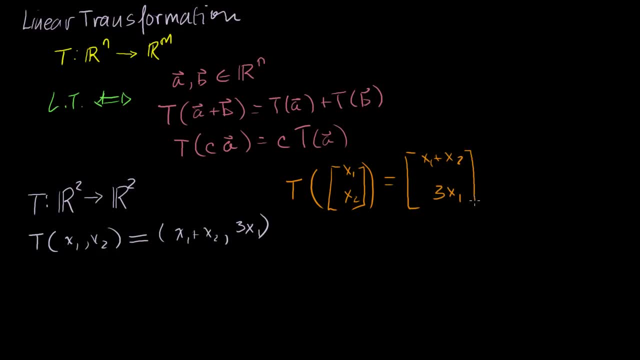 component of the new vector would be 3x1.. That's a completely legitimate way to express our transformation. And the third way, which I never see, but to me it kind of captures the essence of what a transformation is. It's just a mapping or it's just a function. 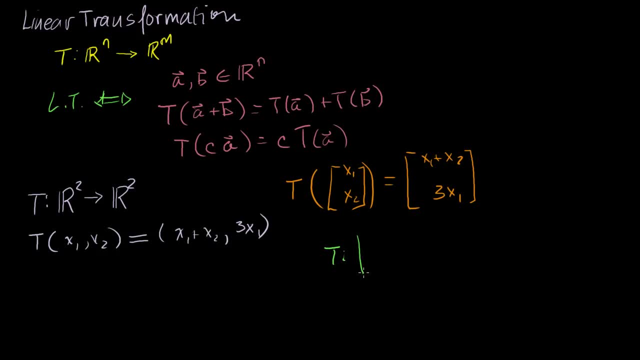 We could say that the transformation is a mapping from any vector in R2 that looks like this: x1, x2, to- and I'll do this notation- to, a vector that looks like this: x1 plus x2, and then 3x1. 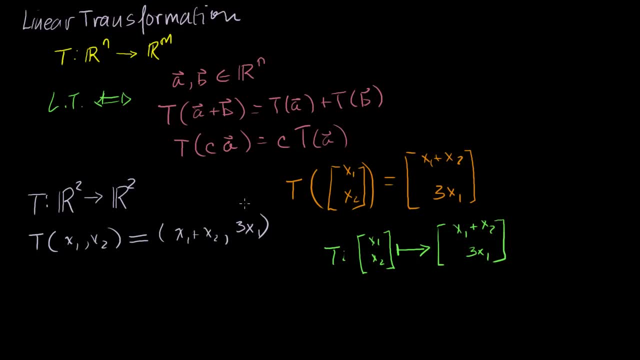 All of these statements are equivalent, But our whole point of writing this is to figure out whether T is linearly independent. So I want to- sorry, not linearly independent- whether it's a linear transformation. I was so obsessed with linear independence for so many. 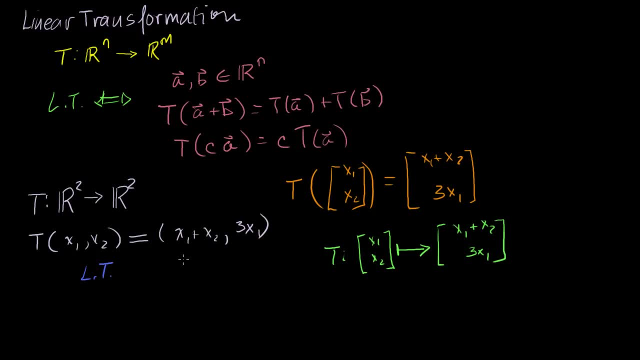 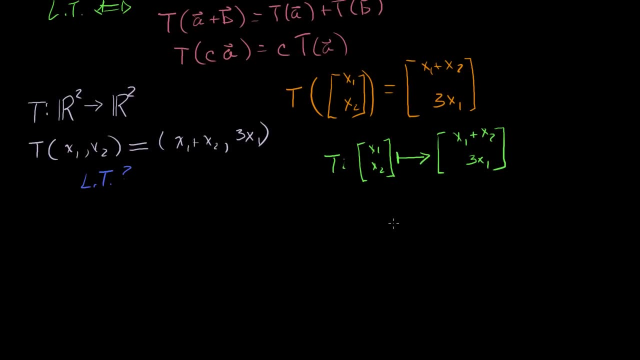 videos. it's hard to get it out of my brain in this one Whether it's a linear transformation. So let's test our two conditions. I have them up here. So let's take T of. let's say I have two vectors, a and b. 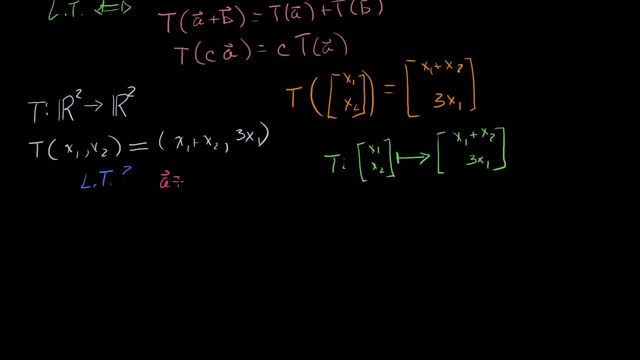 They're members of R2.. So let me write it: a is equal to a1, a2.. And b is equal to b1, b2.. Sorry, that's not a vector. I have to make sure that those are scalars. 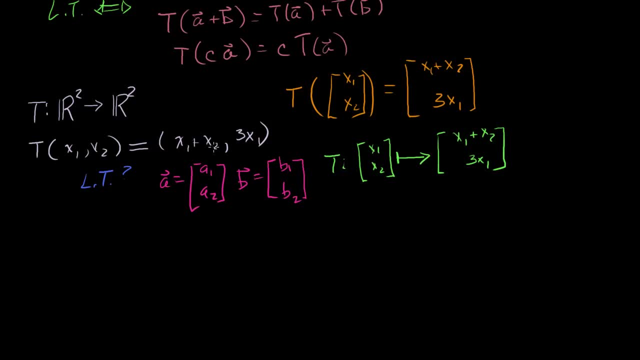 These are the components of a vector And b2.. So what is vector a plus vector b? Brain's malfunctioning, All right. Well, you just add up their components. This is the definition of vector addition. So it's a1 plus b1.. 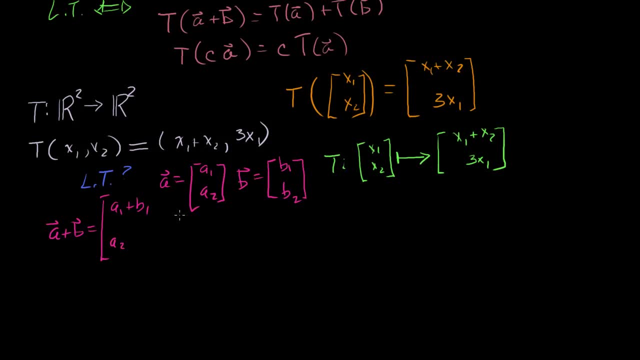 Add up the first components And the second components is just the sum of each of the vector. second components: a2 plus b2.. Nothing new here. But what is the transformation of this vector? So the transformation of vector a plus vector b we. 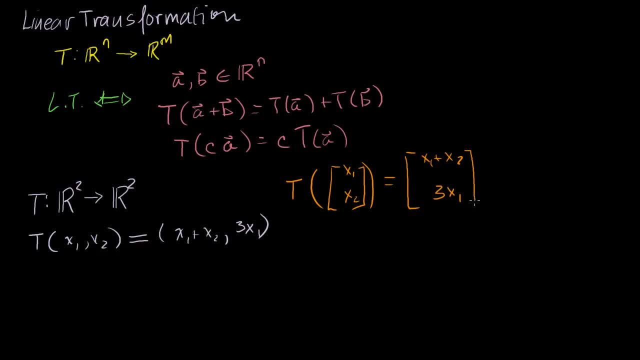 component of the new vector would be 3x1.. That's a completely legitimate way to express our transformation. And the third way, which I never see, but to me it kind of captures the essence of what a transformation is. It's just a mapping or it's just a function. 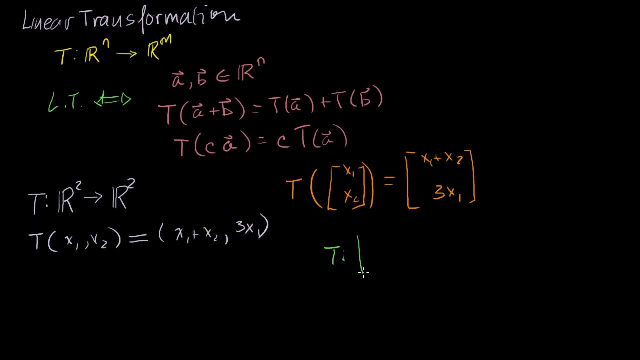 We could say that the transformation is a mapping from any vector in R2 that looks like this: x1, x2 to- and I'll do this notation- to a vector that looks like this: x1 plus x2, and then 3x1.. 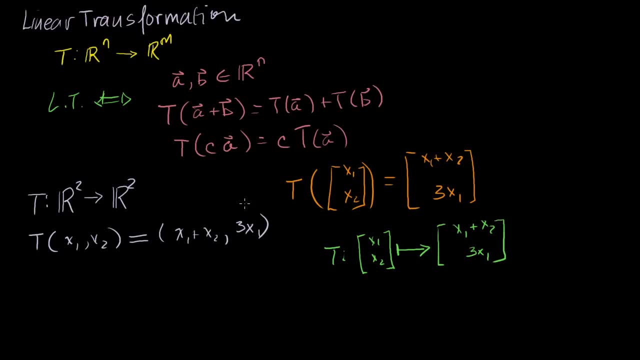 All of these statements are equivalent, But our whole point of writing this is to figure out whether T is linearly independent. So I want to- sorry, not linearly independent- whether it's a linear transformation. I was so obsessed with linear independence for so many. 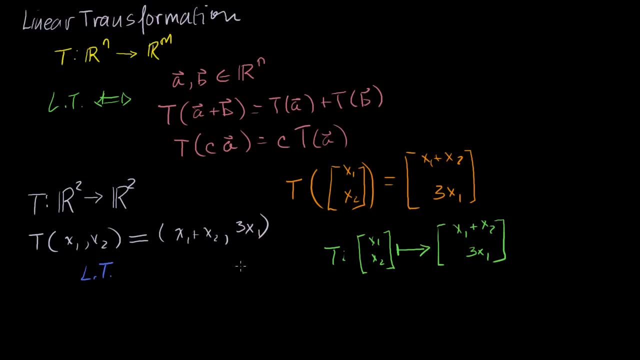 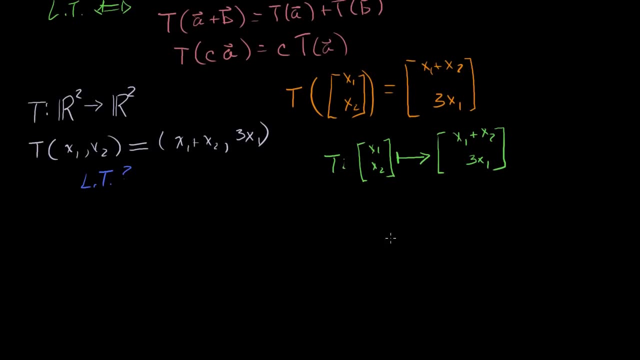 videos. it's hard to get it out of my brain in this one Whether it's a linear transformation. So let's test our two conditions. I have them up here. So let's take T of. let's say I have two vectors, a and b. 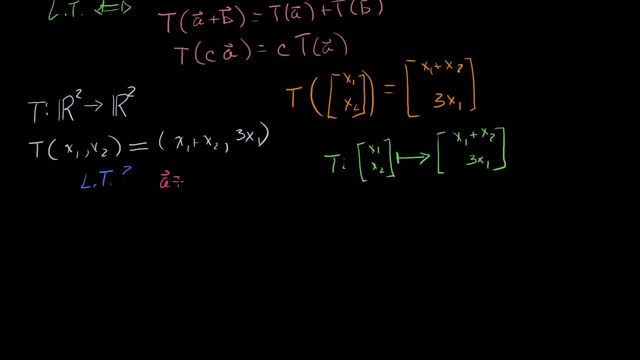 They're members of R2.. So let me write it: a is equal to a1, a2.. And b is equal to b1, b2.. Sorry, that's not a vector. I have to make sure that those are scalars. 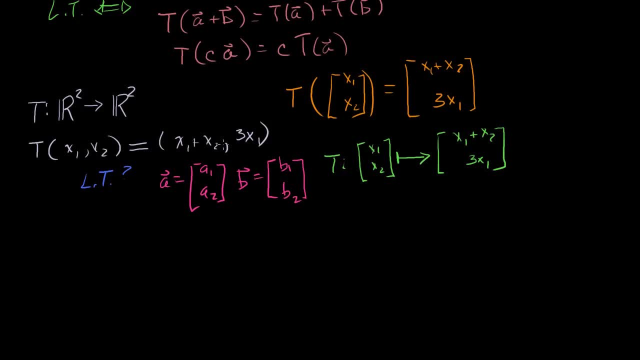 These are the vectors, The components of a vector And b2.. So what is a1 plus b? Sorry, what is vector a plus vector b? Brain's malfunctioning, All right, Well, you just add up their components. This is the definition of vector addition. 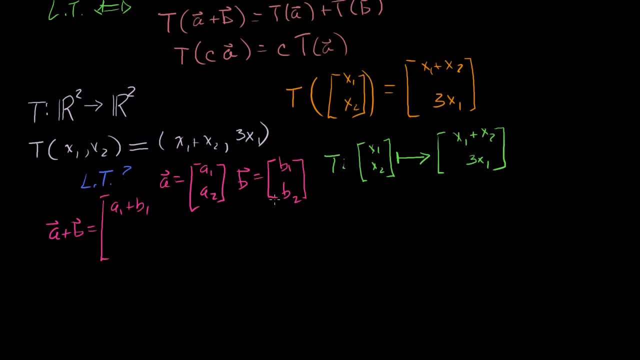 So it's a1 plus b1.. Add up the first components And the second components is just the sum of each of the vector. second components: a2 plus b2.. Nothing new here. But what is the transformation of this vector? So the transformation. 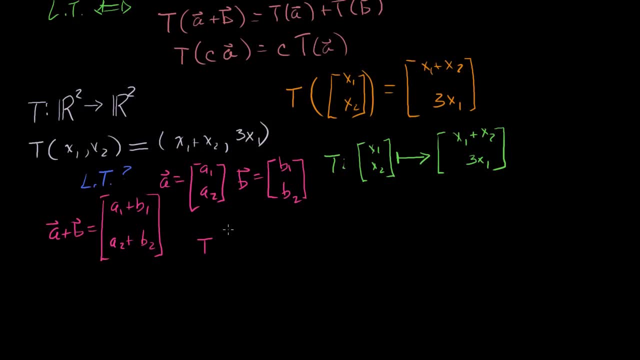 The transformation of vector a plus vector b. We could write it like this: That would be the same thing as the transformation of this vector, which is just a1 plus b1 and a2 plus b2, which we know. it equals a vector. 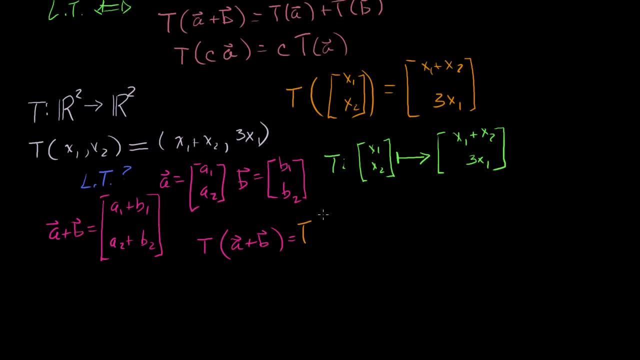 could write it like this: That would be the same thing as the transformation of this vector, which is just a1 plus b1 and a2 plus b2, which we know. it equals a vector. It equals this vector, Where what we do is for the first component. here we add: 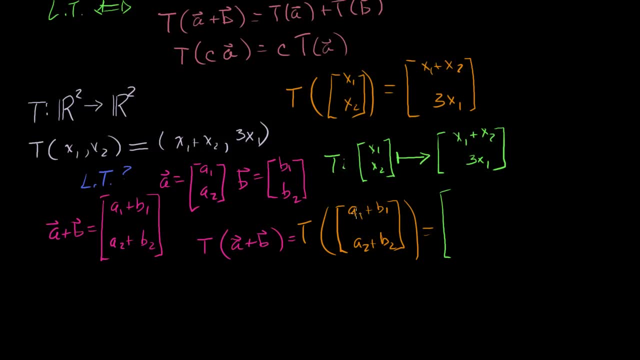 up the two components on this side. So the first component here is going to be these two guys added up, So it's a1 plus a2 plus b1 plus b2.. And then the second component, by our transformation or our function definition, is just three times the first. 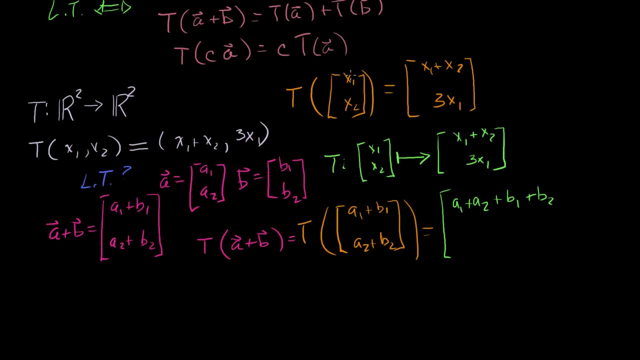 component in our domain, I guess you could say. So it's three times the first one, So it's going to be three times this first guy. So it's 3a1 plus 3b1.. Fair enough. Now what is the transformation individually of a and b? 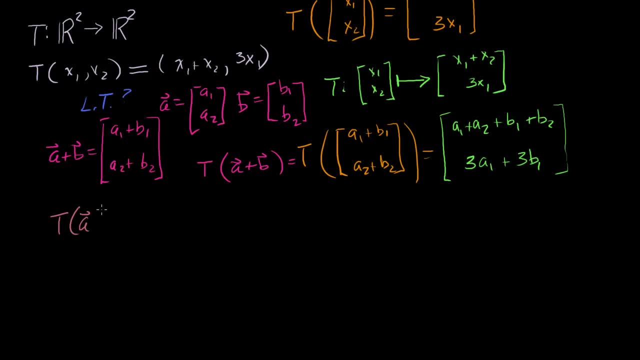 So the transformation of a is equal to the transformation of a. let me write it this way: is equal to the transformation of a1, a2 in brackets. That's another way of writing vector a. And what is that equal to? That's our definition of our transformation, right up here. 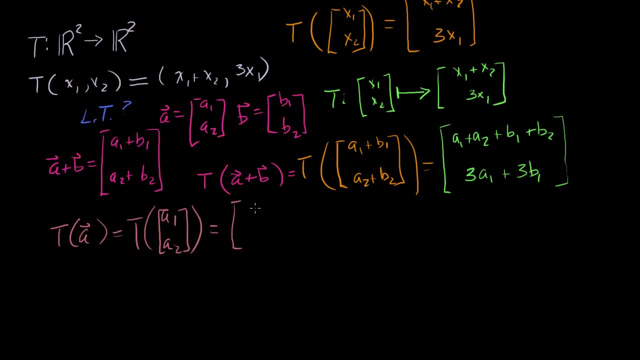 So this is going to be equal to the vector a1 plus a2, and then 3 times a1.. Just come straight out of this definition. I essentially just replaced an x with a's By the same, I guess, argument. what is the? 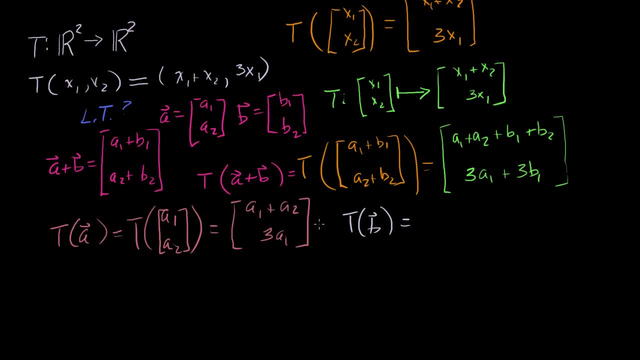 transformation of our vector b. Well, it's just going to be the same thing, with the a's replaced by the b's. So the transformation of our vector b is going to be: b is just b1, b2.. So it's going to be b1 plus b2, and then the second. 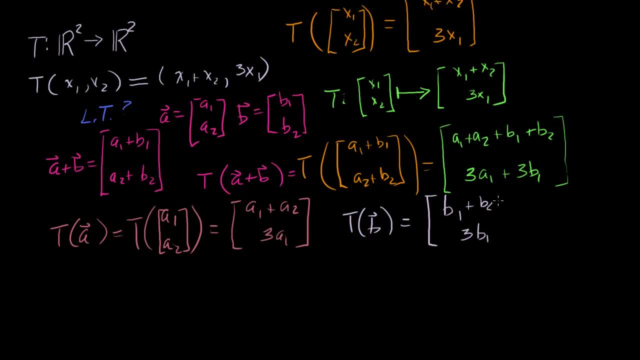 component in the transformation, It will be 3 times b1.. Now what is the transformation of vector a plus the transformation of vector b? What's this vector plus that vector And what is that equal to? Well, this is just pure vector addition, so we just add up. 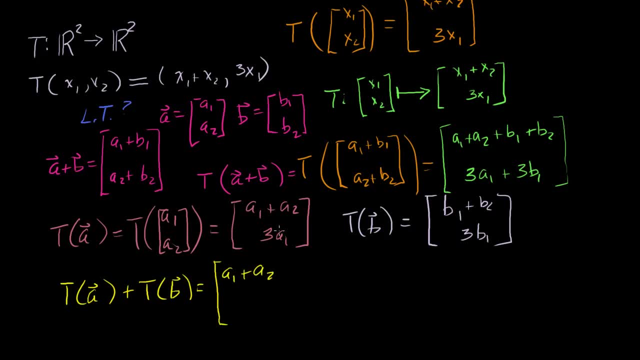 their components. So it's a1 plus a2 plus b1 plus b2.. That's just that component plus that component. And the second component is 3a1 plus b1 plus b2 plus b2.. That's just that component plus that component. 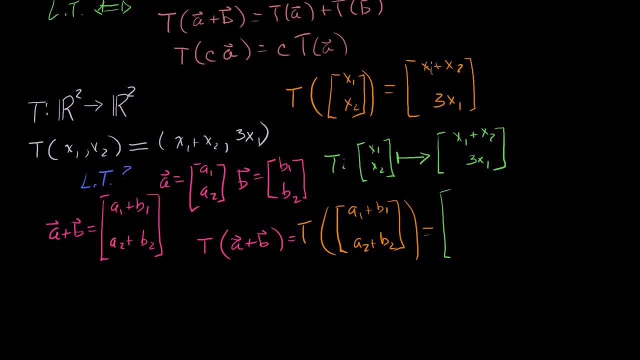 It equals this vector Where what we do is, for the first component here we add up the two components on this side. So the first component here is going to be these two guys added up, So it's a1 plus a2 plus b1 plus b2.. 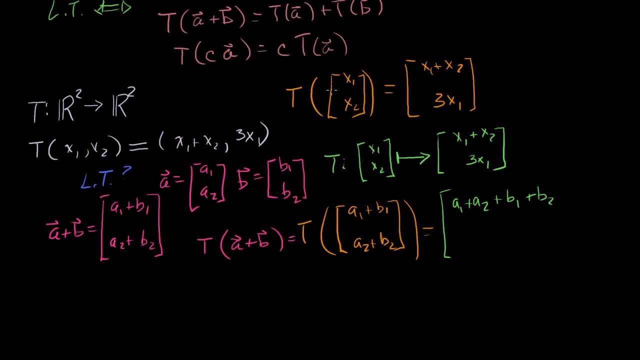 And then the second component, by our transformation or our function definition is just three times the first component in our domain. I guess you could say So it's three times the first one, So it's going to be three times this first guy. 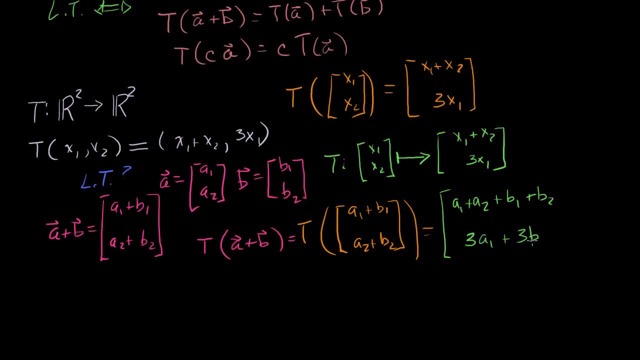 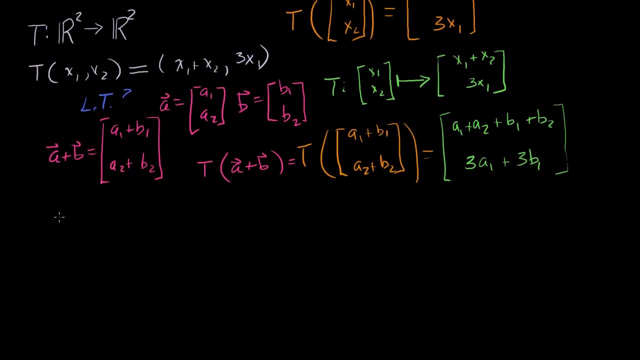 So it's 3a1 plus 3b1.. Fair enough. Now what is the transformation? The transformation individually of a and b. So the transformation of a is equal to the transformation of a. let me write it this way- is equal to the transformation. 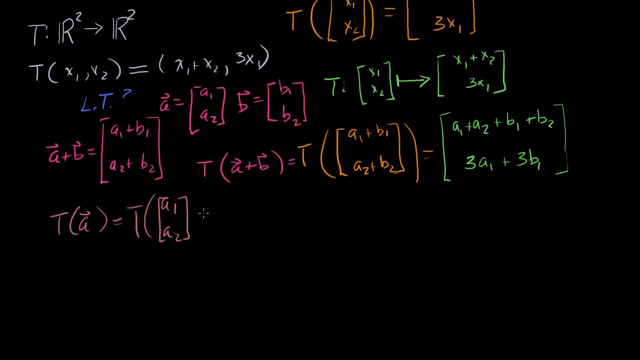 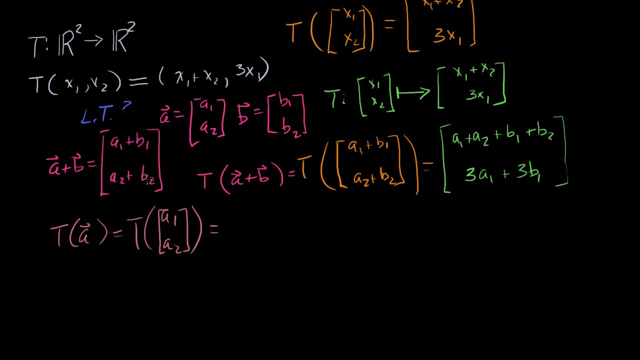 of a1, a2, in brackets. That's another way of writing vector a. And what is that equal to? That's our definition of our transformation right up here. So this is going to be equal to the vector a1, a2, and b2.. 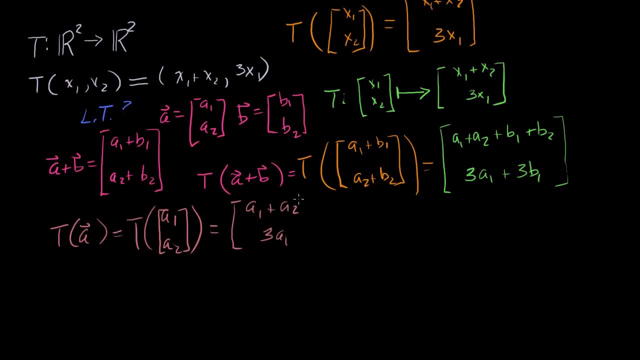 Plus a2.. And then 3 times a1.. Just come straight out of this definition. I essentially just replaced an x with a's By the same, I guess, argument. what is the transformation of our vector b? Well, it's just going to be the same thing with the a's. 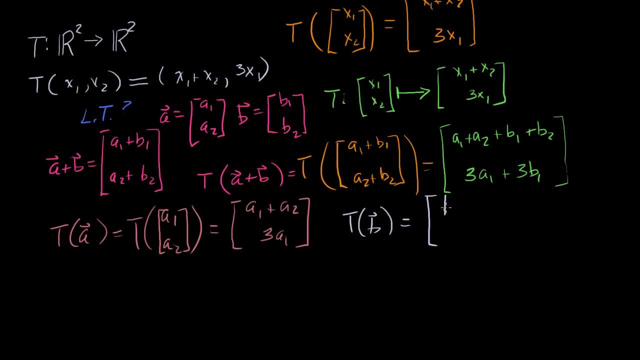 replaced by the b's. So the transformation of our vector b is going to be: b is just b1, b2.. So it's going to be b1 plus b2.. And then the second component in the transformation will be 3 times b1.. 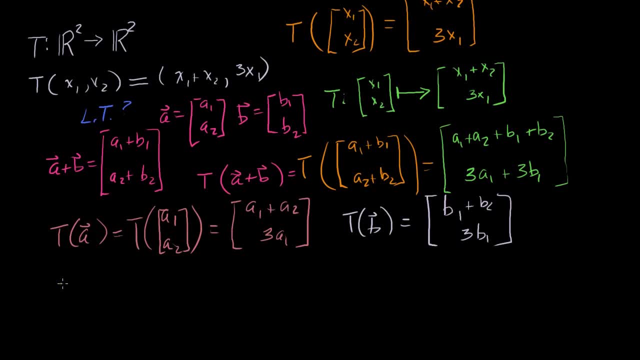 Now, what is the transformation of vector a plus the transformation of vector b? What's this vector plus that vector, And what is that equal to? Well, this is just pure vector addition, So we just add up their components, So it's a1 plus a2 plus b1 plus b2.. 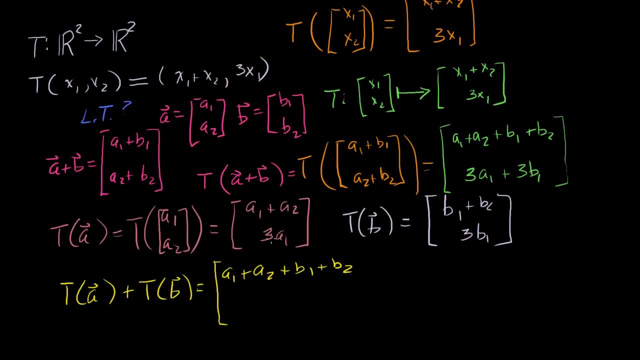 That's just that component plus that component, And the second component is 3a1, and we're going to add it to that, So it's 3a1 plus 3b1.. Now, we just showed you that, if I take the transformation, 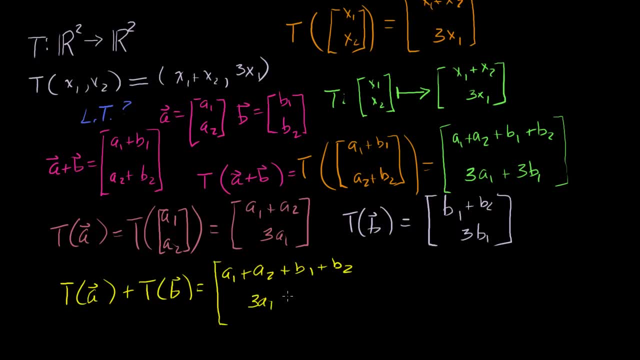 And we're going to add it to that second component. So it's 3a1 plus 3b1.. Now we just showed you that if I take the transformation separately of each of the vectors and then add them up, I get the exact same thing as if I took the vectors and added. 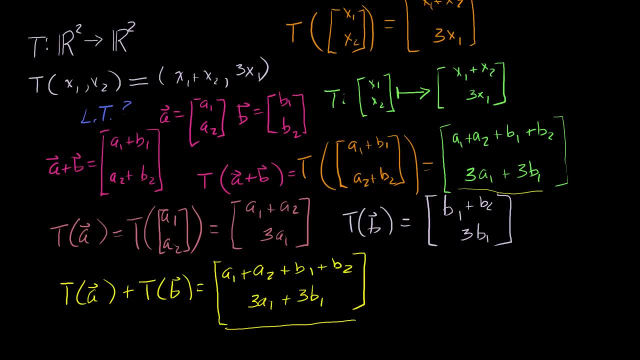 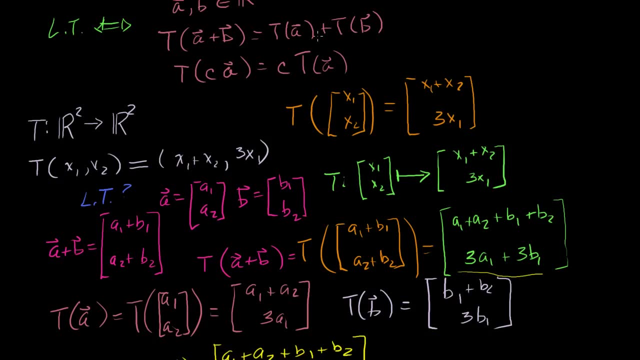 them up first and then took the transformation. So we've met our first criteria, that the transformation of the sum of the vectors is the same thing as the sum of the transformations. Now let's see if this works with the sum of the random scalar. 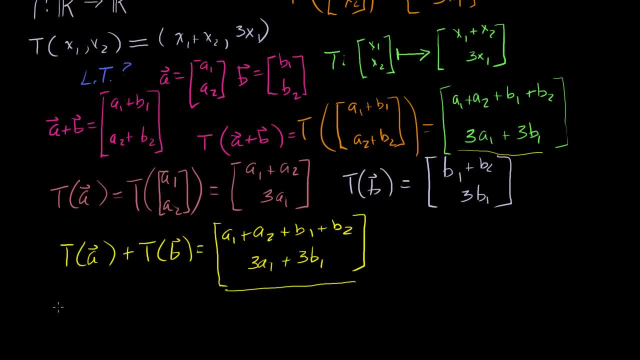 So we know what the transformation of a looks like, but what does ca look like? first of all, I guess that's a good place to start c times. our vector a is going to be equal to c times a1 and then c times a2.. 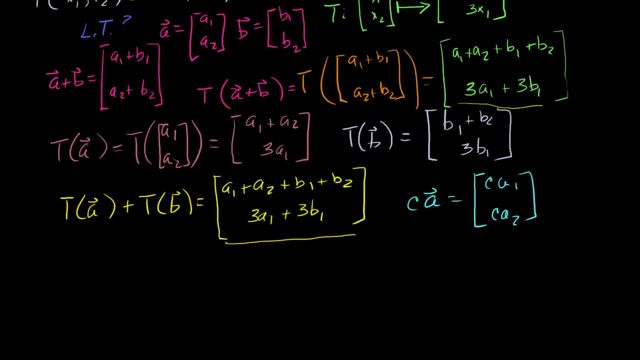 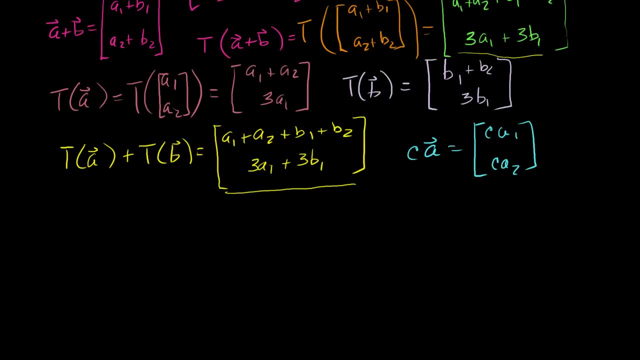 That's our definition of scalar multiplication times a vector. So what's our transformation? Let me go to a new color. What is our? let me do a color I haven't used in a long time- white. What is our transformation of ca going to be? 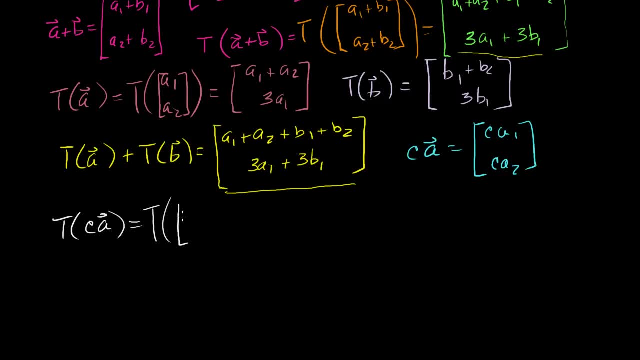 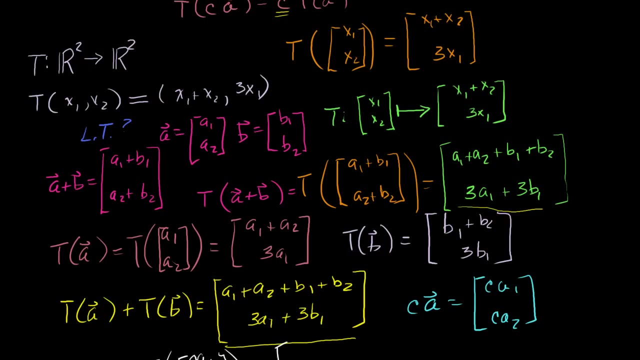 Well, that's the same thing as our transformation of ca1, ca2,, which is equal to a new vector, where the first term- let's go to our definition- is: you sum the first and second components and then the second term is three times the first. 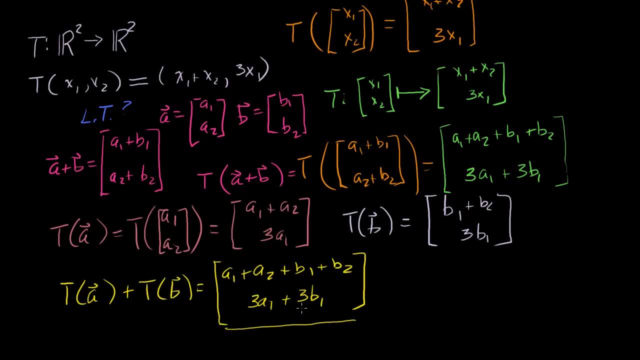 separately of each of the vectors and then add them up, I get the exact same thing as if I took the vectors and added them up first and then took the transformation. So we've met our first criteria, that the transformation of the sum of the vectors is the same thing. 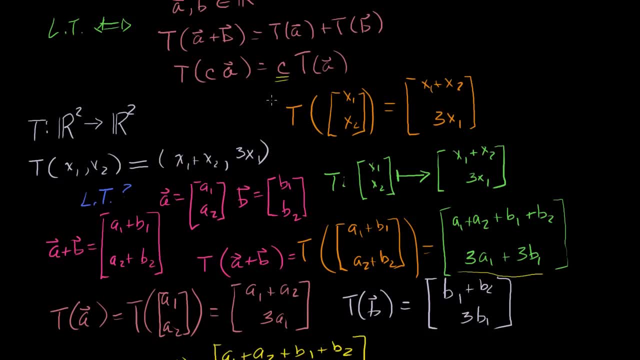 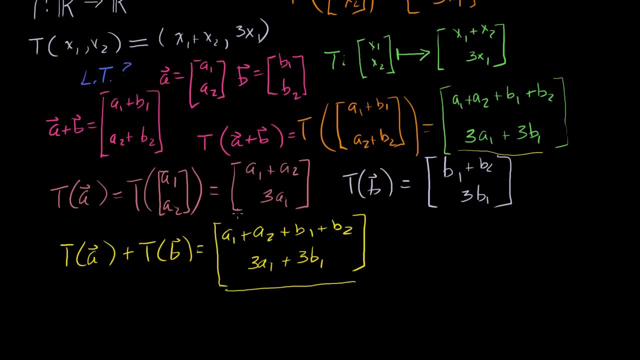 as the sum of the transformations. Now let's see if this works with a random scalar. So we know what the transformation of a looks like. What does c a look like? first of all, I guess that's a good place to start. 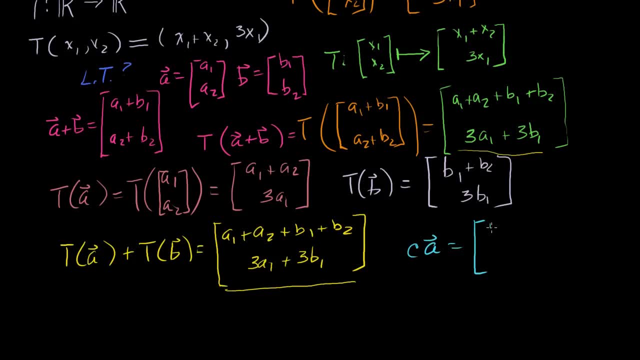 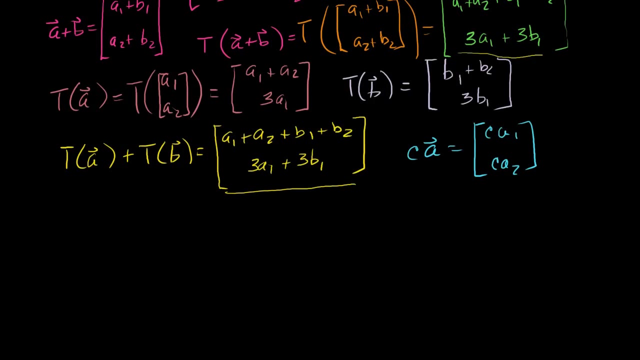 c times our vector. a is going to be equal to c times a1 and then c times a2.. That's our definition of scalar multiplication times a vector. So what's our transformation? Let me go to a new color. What is our? let me do a color I haven't used in a long time. 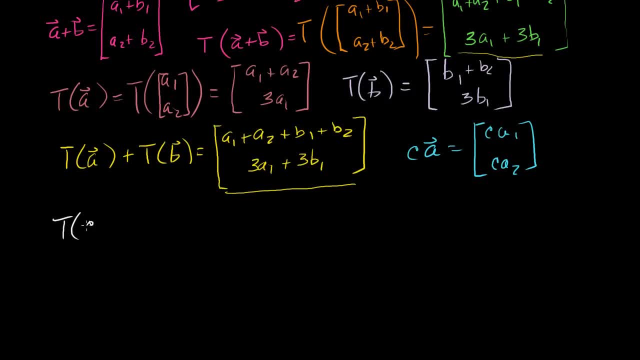 white. What is our transformation Of c a going to be? Well, that's the same thing as our transformation of c a1, c a2, which is equal to a new vector, where the first term- let's go to our definition- is: you sum the first and second components. 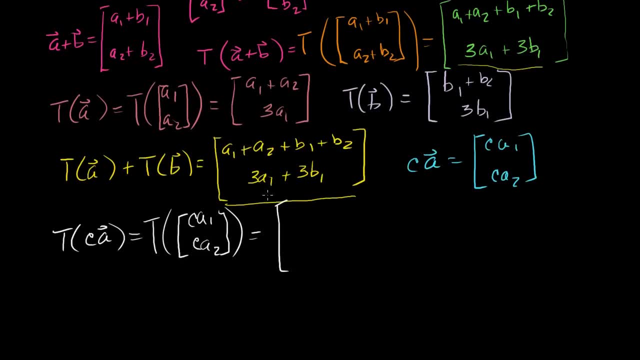 and then the second term is three times the first component, So our first term, you sum them, So it's going to be c a1 plus c a2.. And then our second term is three times our first term, So it's three c a1.. 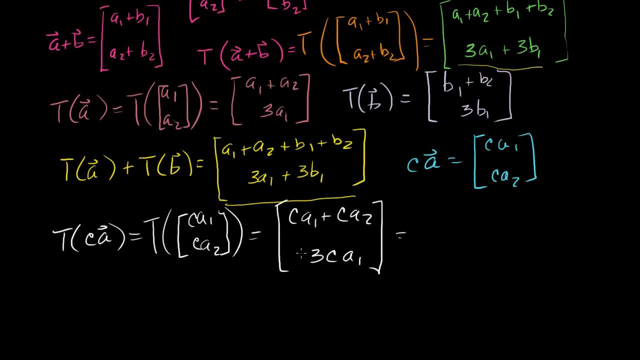 Now, what is this equal to? This is the same thing. We can kind of view it as factoring out the c. This is the same thing as c times the vector a1 plus a2, and then the second component is 3a1.. 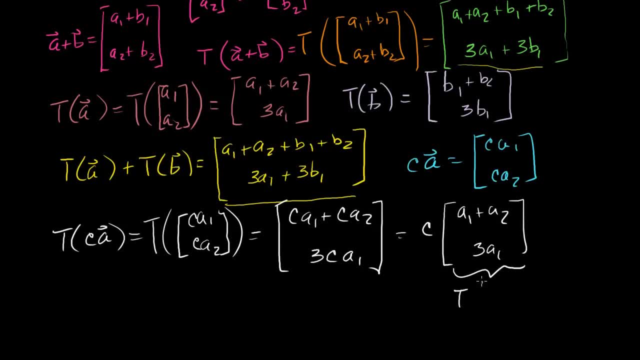 But this thing right here we already saw This is the same thing as the transformation of a, The transformation of a. So just like that, you see that the transformation of c times our vector a. For any vector a, we're going to get a vector a. 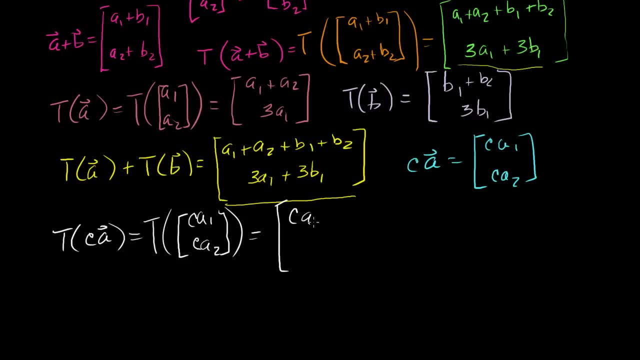 component, So our first term. you sum them so it's going to be ca1 plus ca2.. And then our second term is three times our first term, So it's 3ca1.. Now what is this equal to? 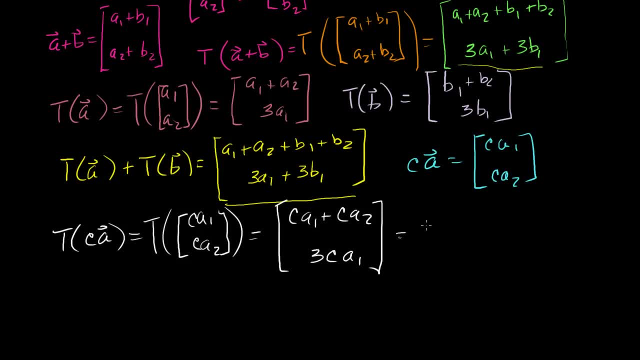 This is the same thing. We can kind of view it as factoring out the c. This is the same thing as c times the vector a1 plus a2.. And then the second component is 3a1.. But this thing right here we already saw this is the same. 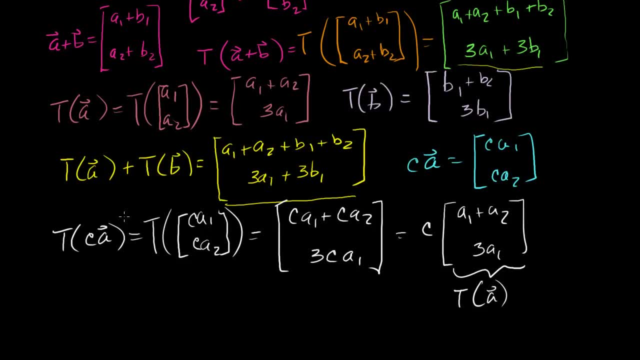 thing as the transformation of a Transformation of a. So just like that, you see that the transformation of c times our vector a. for any vector a in R2, anything in R2 can be represented this way. it's the same thing as c times. 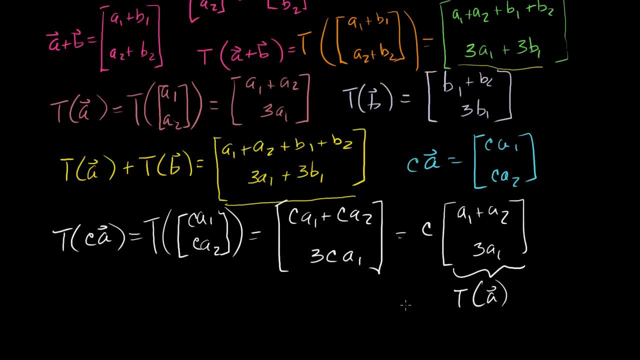 So what's the transformation of c times vector a? What's the transformation of a? Okay, So what's the transformation of c times vector a? A in R2, anything in R2 can be represented this way. It's the same thing as C times. the transformation of A. 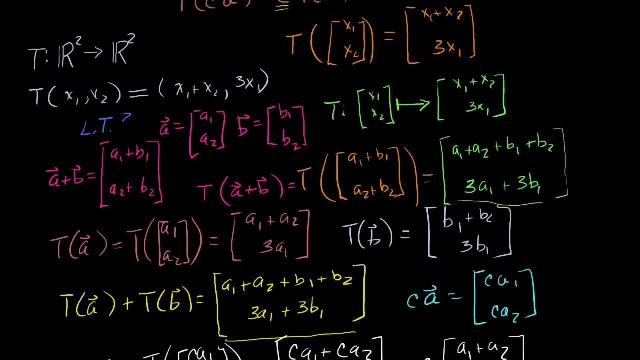 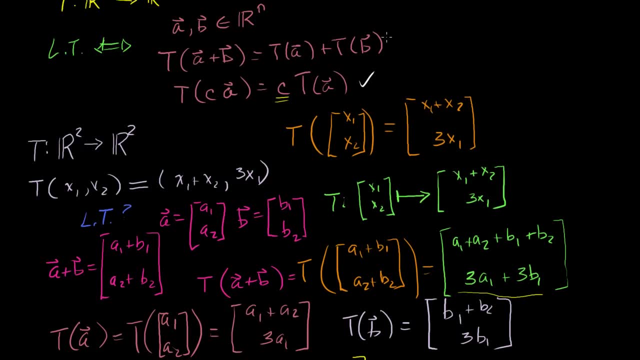 the transformation of a. So we've met our second condition, that it doesn't that when you. well, I just stated it, so I don't have to restate it. So we meet both conditions, which tells us that this is a. 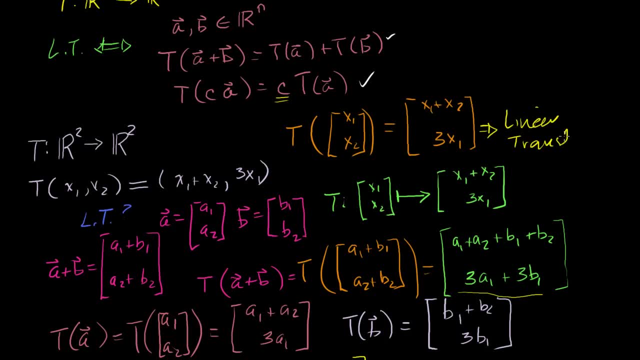 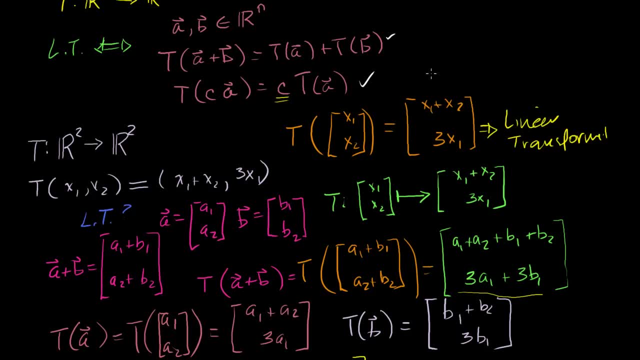 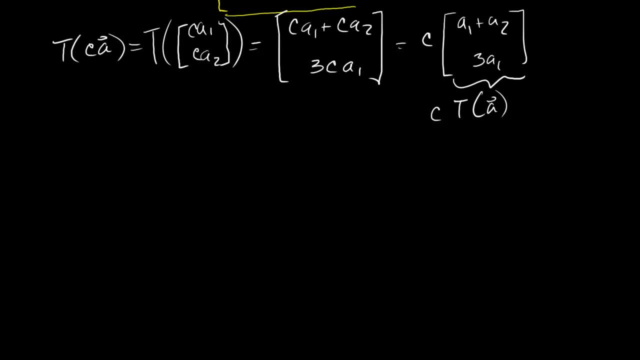 And here I'll do a very simple example. Let me define my transformation And just to make it, oh, let me do one, Let me make it. let me see, Let me define a transformation. Well, I'll do it from R2 to R2, just to kind of compare the two. 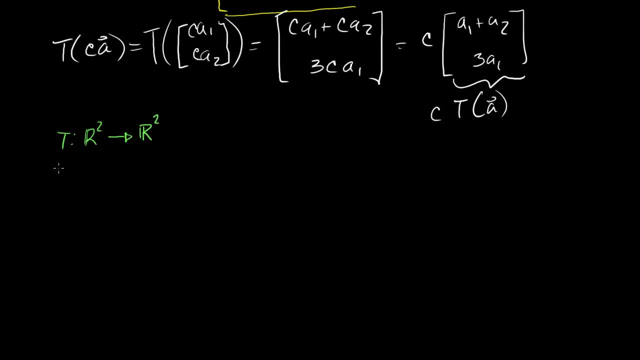 I could have done it from r to r if I wanted a simpler example, but I'm going to define my transformation. Let's say my transformation of the vector x1, x2.. Let's say it is equal to. let me just say x1 squared and. 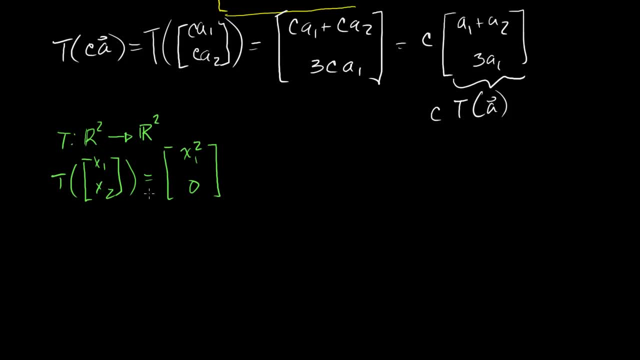 then 0, just like that. Let me see if this is a linear transformation. So the first question is: what's my transformation of a vector a? So my transformation of a vector a, where a is just the same a that I did before, it would look like this: 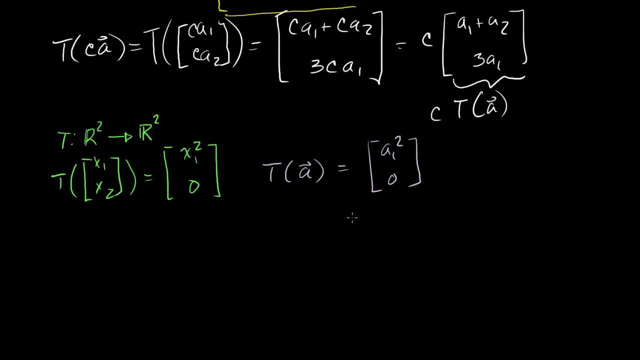 It would look like a1 squared and then a 0. Now, what would be my transformation if I took c times a? Well, this is the same thing as c times a1 and c times a2.. And, by our transformation definition, if I take the 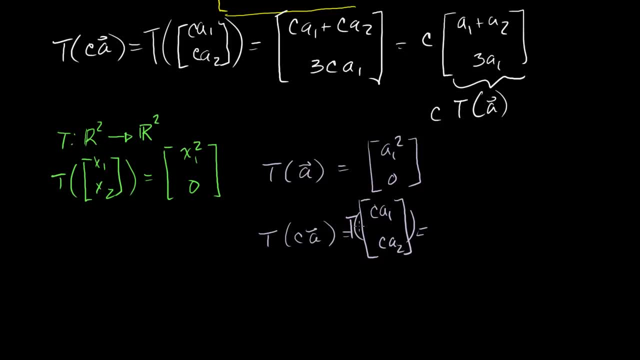 transformation of c times, of this thing right here, because I'm taking the transformation on both sides and by our transformation definition this will just be equal to a new vector that would be in our codomain where the first term is just the first term of our input squared. 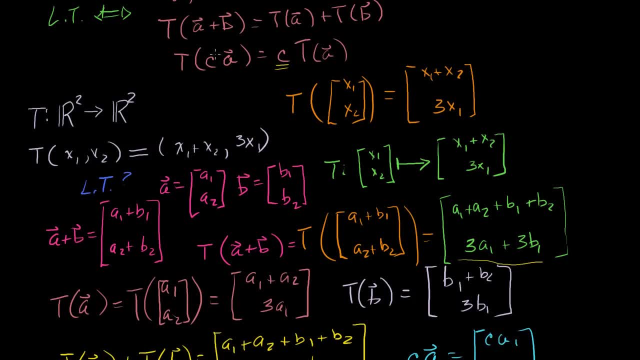 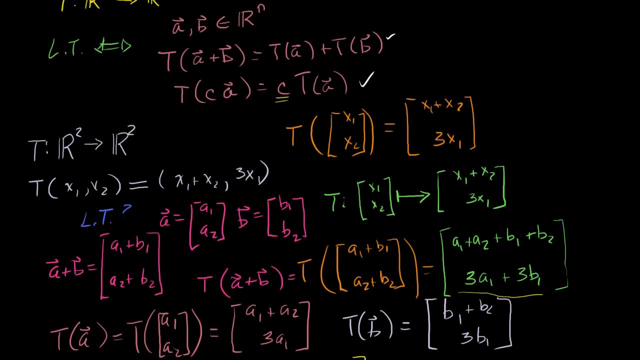 So we've met our second condition. Well, I just stated it so I don't have to restate it. So we meet both conditions, which tells us that this is a linear transformation. And you might be thinking: OK, Sal, fair enough. 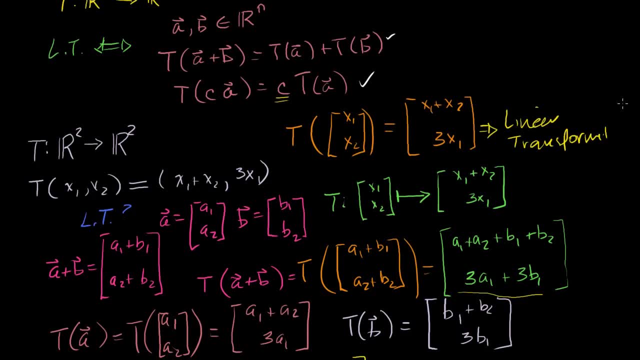 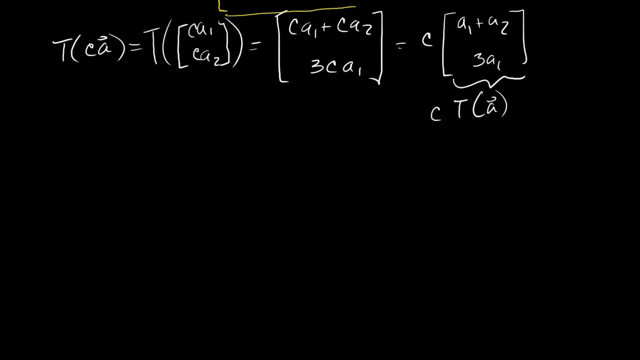 How do I know that all transformations aren't linear? transformations Show me something that won't work. And here I'll do a very simple example. Let me define my transformation. And just to make it, oh, let me define a transformation. Well, I'll do it from R2 to R2, just to. 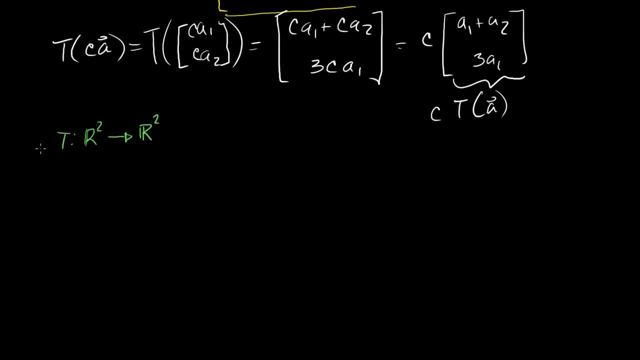 kind of compare the two. I could have done it from R to R if I wanted a simpler example, but I'm going to define my transformation, Let's say my transformation of the vector X1, X2.. Let's say it is equal to, let me just say, x1 squared and. 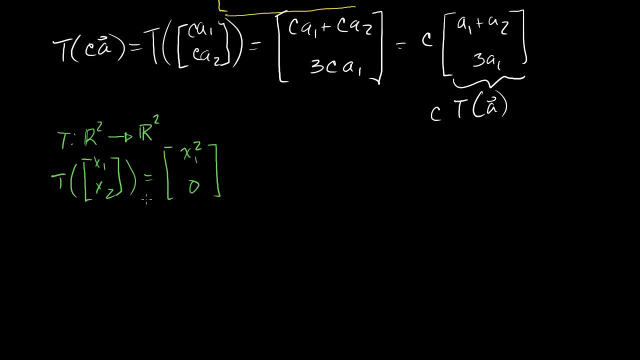 then 0, just like that. Let me see if this is a linear transformation. So the first question is: what's my transformation of a vector A? So my transformation of a vector A where A is just the same A that I did before. 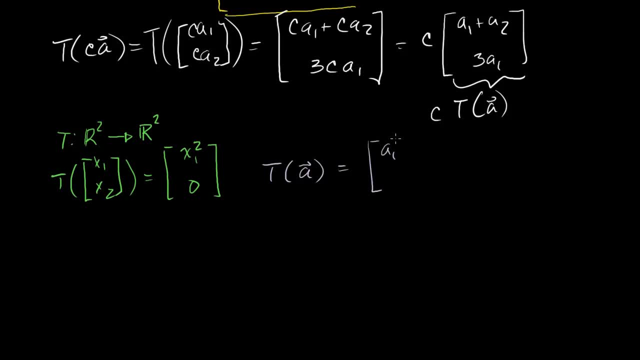 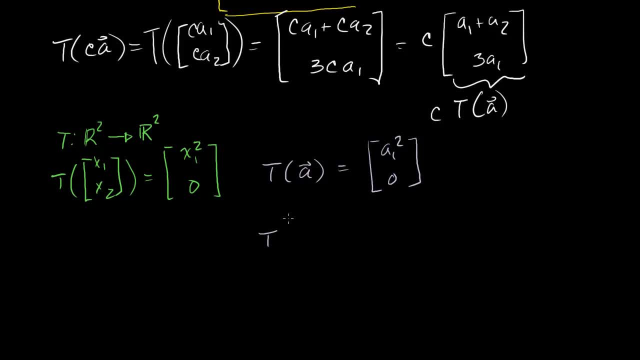 Now, what would be my transformation if I took c times a? Well, this is the same thing as c times a1, and c times a2.. And by our transformation definition, if I take the transformation of c times of this thing right here, because 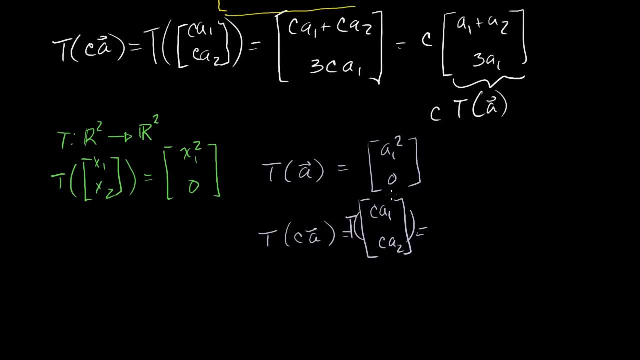 I'm taking the transformation on both sides and by our transformation definition this will just be equal to a new vector that would be in our codomain, where the first term is just the first term of our input squared, So it's CA1 squared and the second term is 0.. 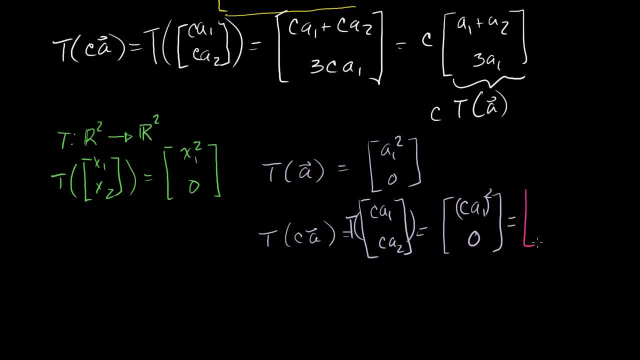 What is this equal to? Let me switch colors. This is equal to C squared A1 squared, and this is equal to 0.. Now let's see if we can factor out. well, if we can assume that C does not equal 0,, this would be equal to what? 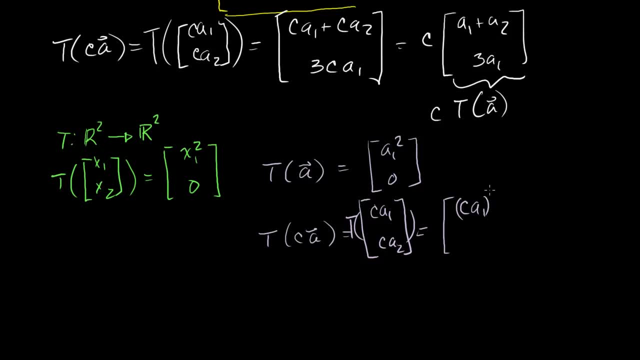 So it's ca1 squared, and the second term is 0.. What is this equal to? Let me switch colors. This is equal to c squared, a1 squared, and this is equal to 0.. Now let's see if we can factor out. 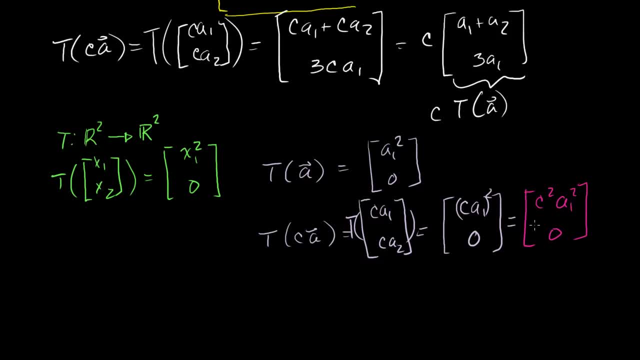 Well, if we can assume that c does not equal 0,, this would be equal to what? Actually, it doesn't even matter, We don't even have to make that assumption. So this is the same thing. This is equal to c squared times the vector a1 squared 0,. 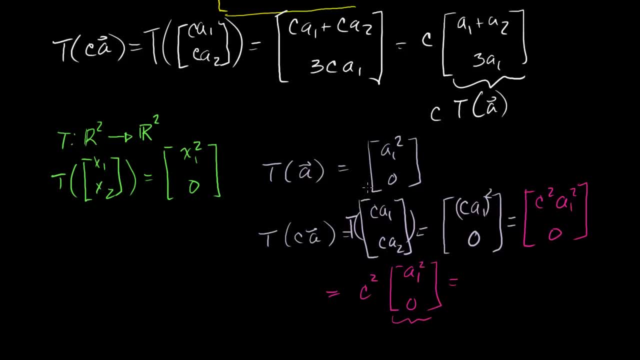 which is equal to c squared a1 squared Equal to what This expression right here is the transformation of a. So this is equal to c squared times the transformation of a. Let me do it in the same color Times: the transformation of a. 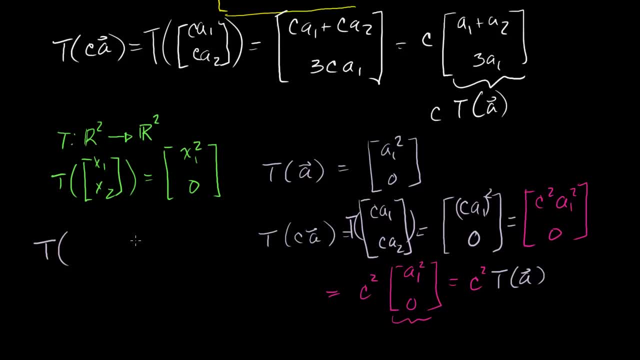 So what I've just showed you is, if I take the transformation of a vector being multiplied by a scalar quantity first, that that's equal to: for this t, for this transformation that I've defined right here, that's equal to c squared times the transformation of a. 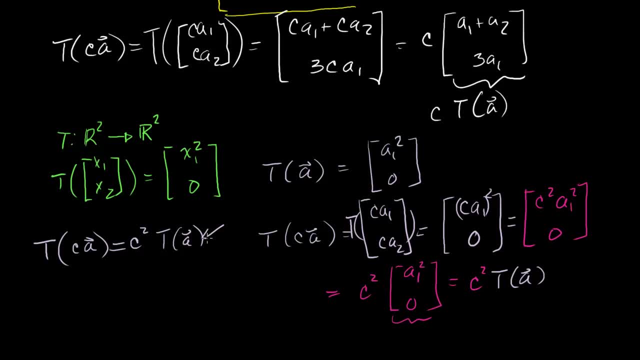 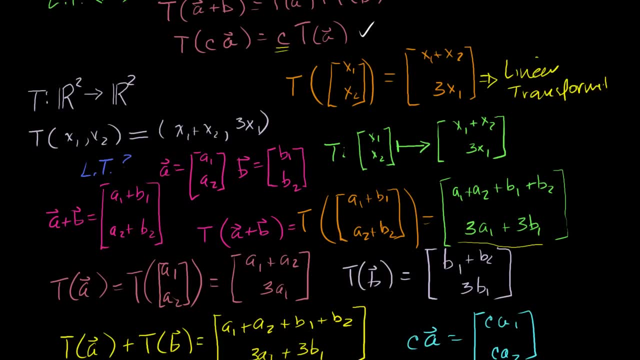 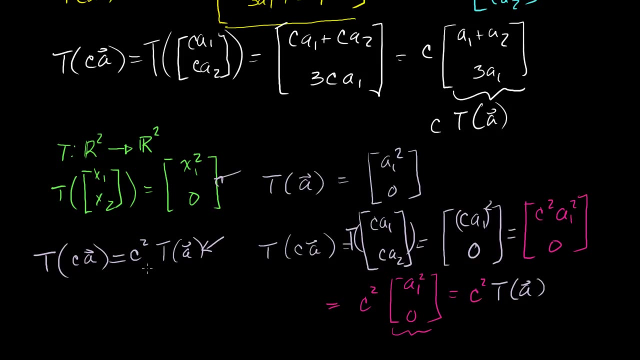 And clearly, this statement right here, for this choice of transformation conflicts with this requirement for a linear transformation. If I have a c here, I should see a c here, But in our case, I have a c here and I have a c squared. 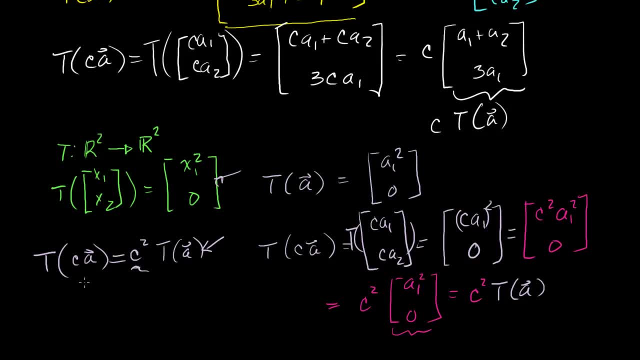 here so clearly. this negates that statement. So we're definitely not dealing. so this is not a linear transformation. And just to get a gut feel, if you're just looking at something, whether it's going to be a linear transformation or not, if the transformation just involves linear, 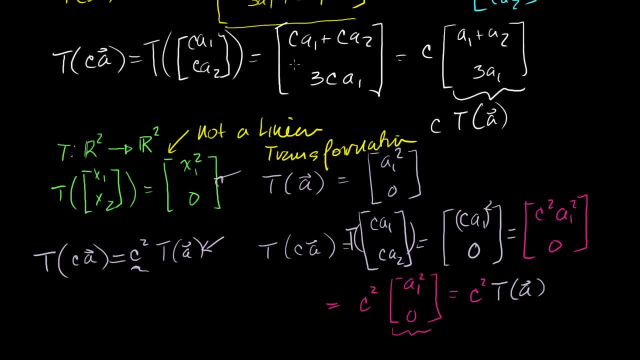 combinations of the different components of the inputs, you're probably dealing with a linear transformation. If you start seeing things where the components start getting multiplied by each other, or you start seeing squares or exponents, you're probably not dealing with a linear transformation. 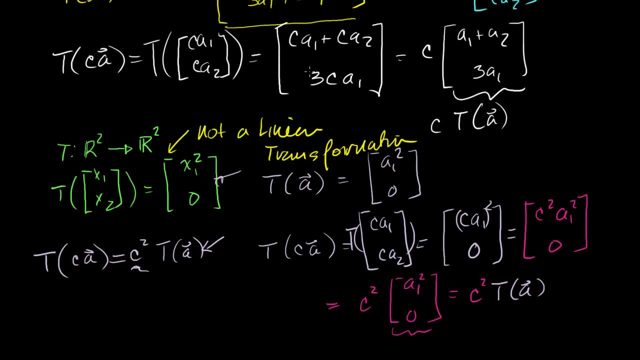 And then there are some functions that might be in a bit of a gray area, But it tends to be just linear combinations are going to deal, lead to a linear transformation, But hopefully that gives you a good sense of things and this leads up to what I think is one of the neatest outcomes in the next video. 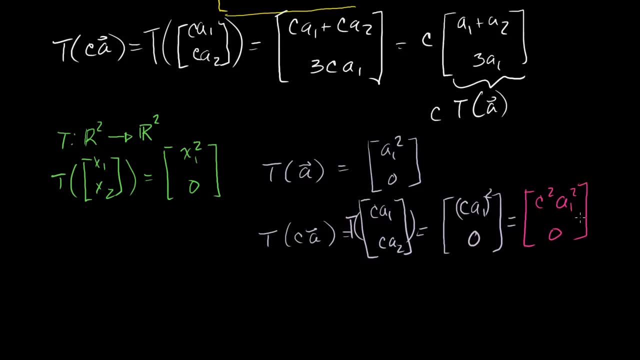 Actually, it doesn't even matter. We don't even have to make that assumption. So this is the same thing. This is equal to C squared times the vector A1 squared 0, which is equal to what This expression right here is the transformation of A. 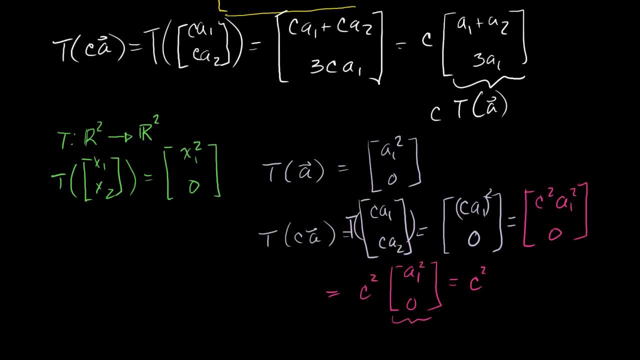 So this is equal to C squared times the transformation of A. Let me do it in the same color Times: the transformation Times, the transformation of A. So what I've just showed you is if I take the transformation of a vector being multiplied by a scalar quantity. first, 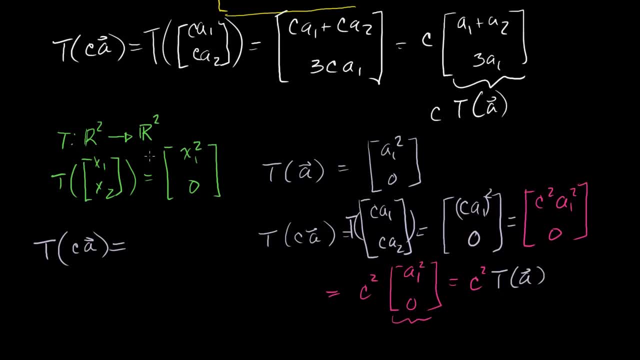 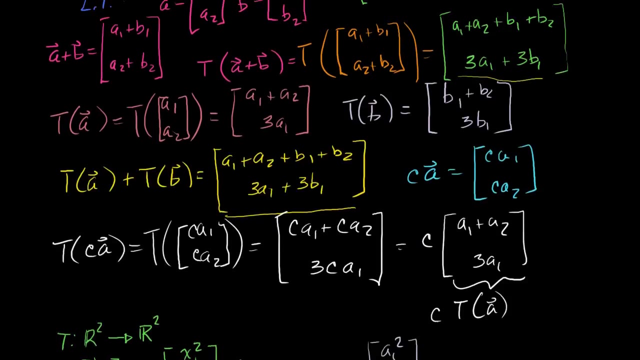 that that's equal to: for this T, for this transformation that I've defined right here, that's equal to C squared times the transformation of A. And clearly, this statement right here, for this choice of transformation, conflicts with this requirement for a linear. 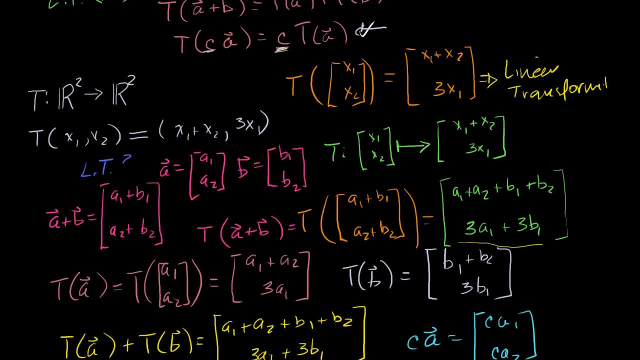 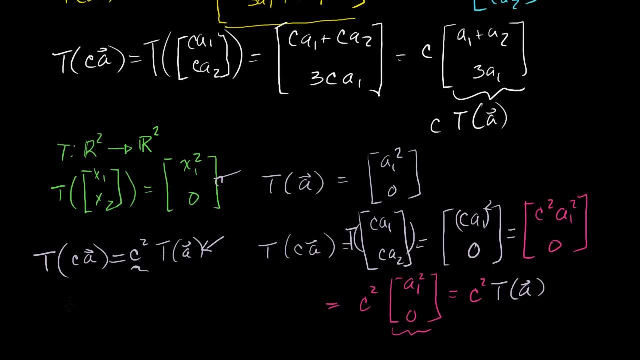 transformation. If I have a C here, I should see a C here. But in our case I have a C here and I have a C squared here. So clearly this negates that statement. So we're definitely not dealing. So this is not a linear transformation. 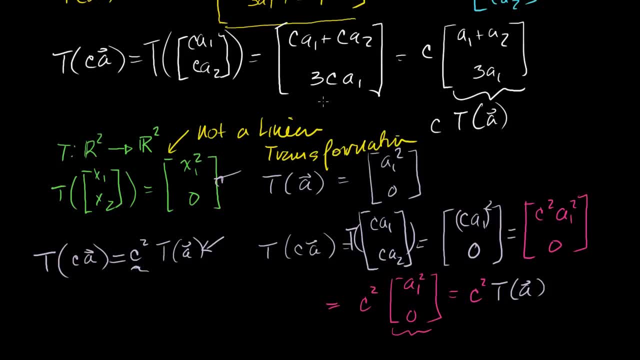 And just to get a gut feel, if you're just looking at something, whether it's going to be a linear transformation or not. If the transformation just involves linear combinations of the different components of the input, You're probably dealing with a linear transformation. 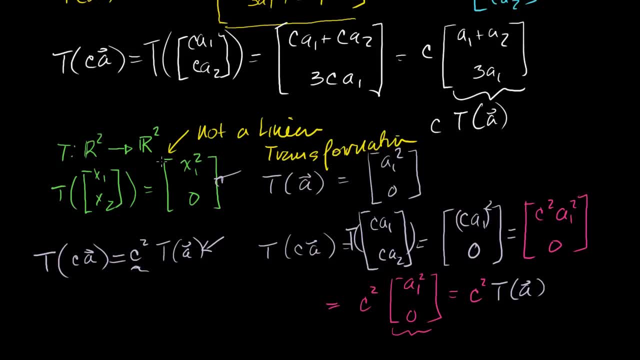 If you start seeing things where the components start getting multiplied by each other, or you start seeing squares or exponents, you're probably not dealing with a linear transformation. And then there are some functions that might be in a bit of a gray area.